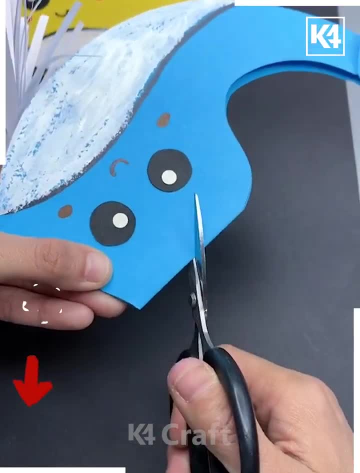 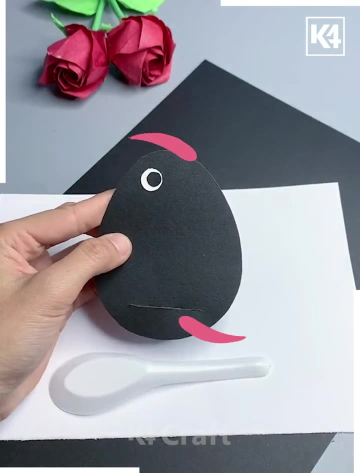 less time consuming. all you require is just colorful sheets of the paper glues. you also require toothpick scissors for the cutting. just go for this one. penguins are the birds that are found in the arctic region, and they are able to survive in the extreme cold conditions. today, we 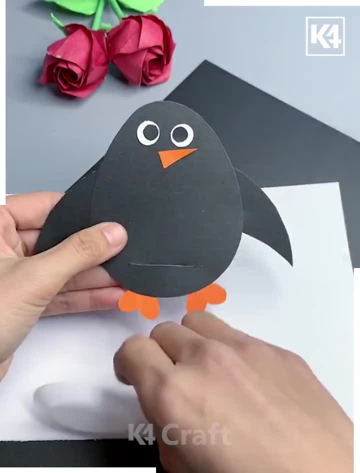 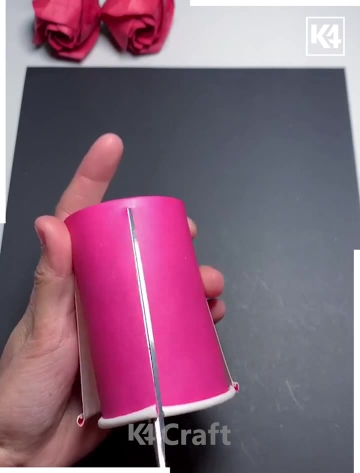 are going to make the paper penguin. for this we may require the black sheet of the paper and a spoon. this is so nice. it's time to make an octopus. for this, we are taking the disposable cup and we are just making the strips out of it. after that, we are just creating the curls that will represent. 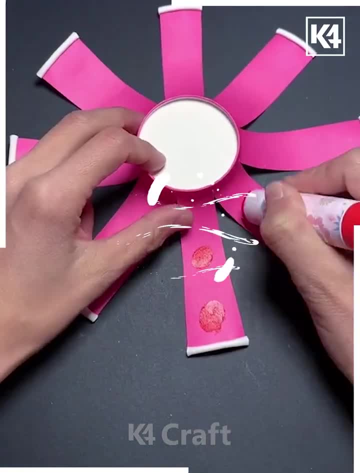 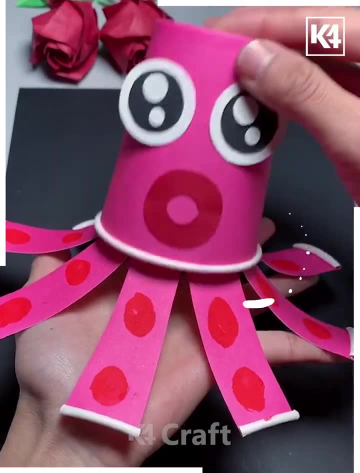 the tentacles of the octopus with the help of the marker. then you just have to add further details, actually patterns of the tentacles, and add the other areas and the features of this octopus. this activity is very simple and it's best suitable for the small kids. for this we are. 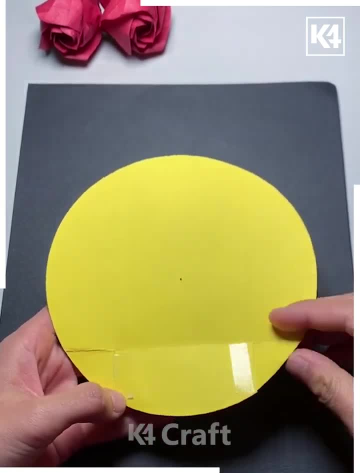 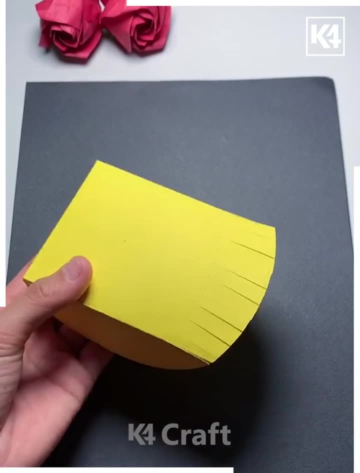 taking this yellow sheet of the paper and we are just trimming it in the circle. look shape after that. we are just creating the other things with the help of the double-sided tip. scissors are also required for creating the tassel type pattern. it will represent the wings. 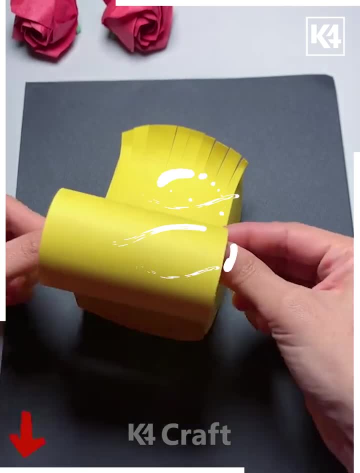 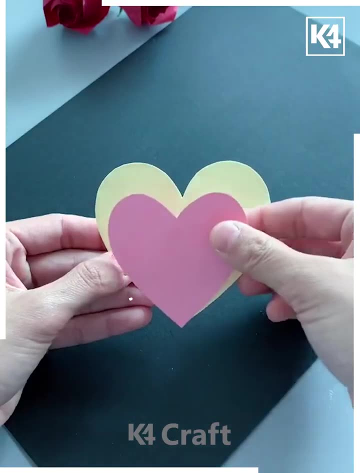 of the duck. this activity is little bit time consuming, but it's very easy. also, don't forget to add the further details, like we are doing here. eyes, and we are placing the b with the help of the disposable spoons. we are going to make the butterfly for wings. we are making use of the 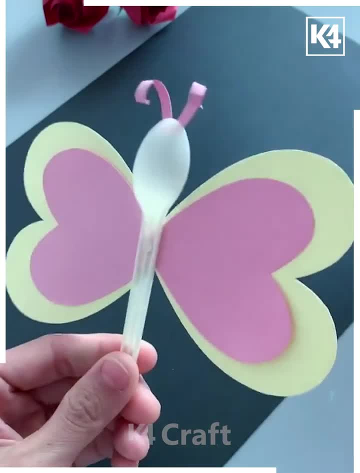 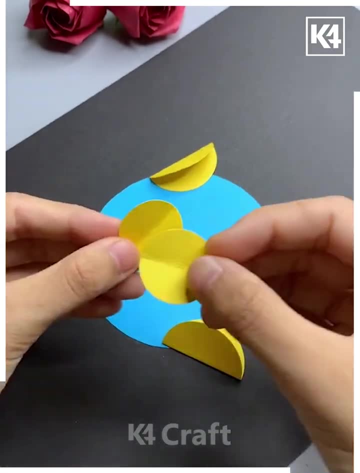 two shades of the paper. this activity is very simple and good for small kids. you may require super glue also for just pasting the antennae. next we are going to make a fish. for this, we are taking the blue sheet that we have trimmed in somewhat circular shape. after that we are just pasting. 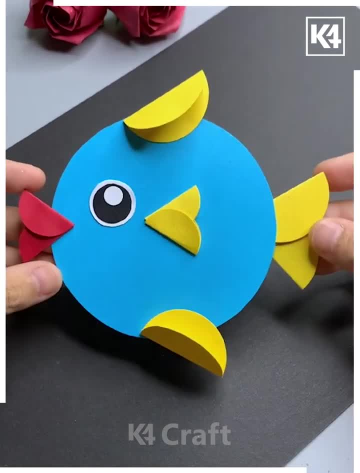 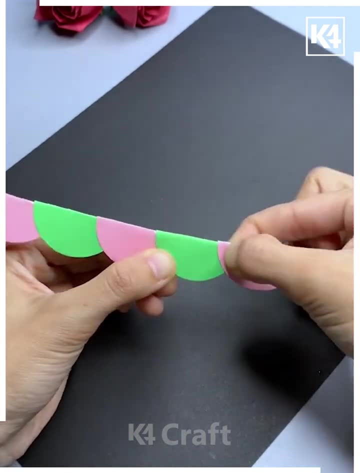 these yellow sheets. these will represent the fins, and the other features are added. this activity is very simple and it's best suitable for the small kids between the age group of six to seven. for this, you just need to punch out the circular sheets and then you just have to. 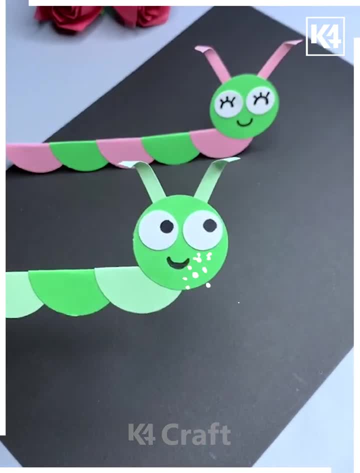 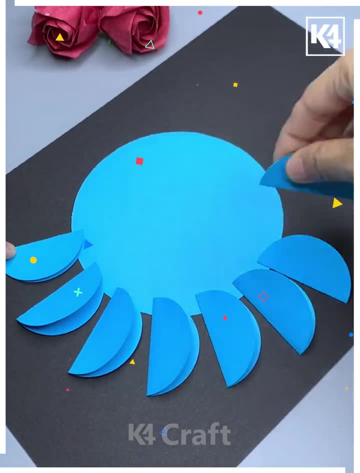 paste them one above the other in the folded form. add the further details. for our next activity, we again require some colorful sheets of paper, and we are going to make a fish for this. we are taking two sheets of the paper and the scissors. we are going to make an octopus for this housey we are. 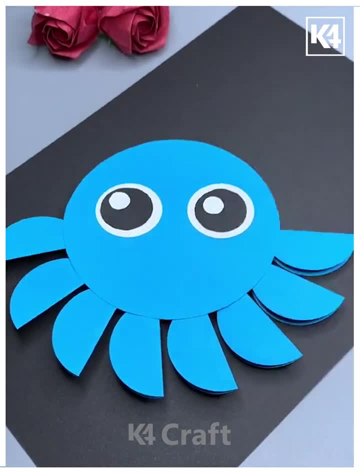 just trimming the circular sheets that we have folded together. these will represent the tentacles. add the further features. thank you for watching.